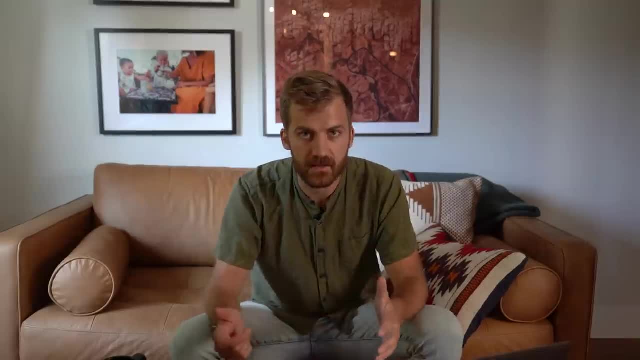 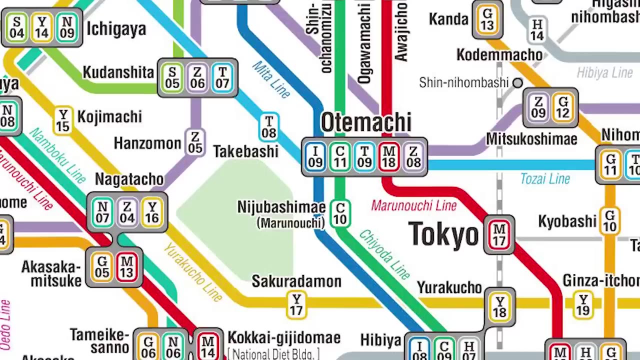 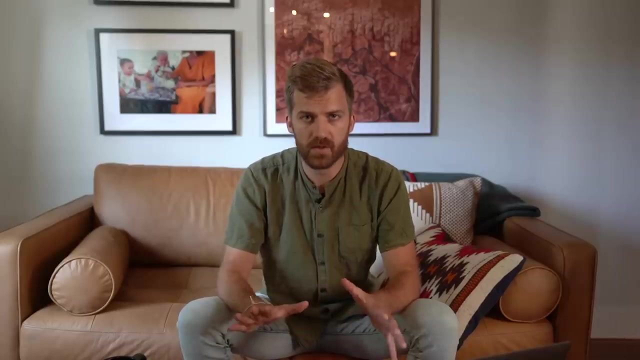 Listen, Tokyo is giant. And the second you start thinking about getting around the city, you're hit with this. Yeah, I know it looks crazy, But I promise this is totally manageable. You can do it, especially if you have a smartphone connected to the internet. We're 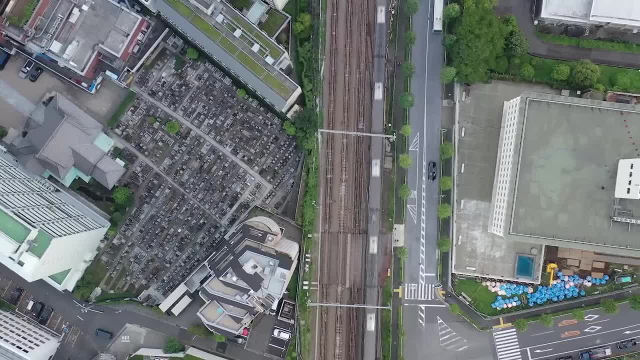 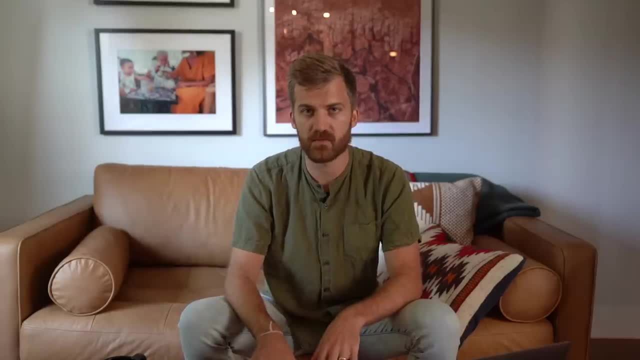 going to go over some of the key concepts that make this world-class transportation system flow, so that you can navigate the city while you're in Tokyo. Luckily, there's some amazing tools on your smartphone that can help you do this, And, at the end of the day, you won't really be. 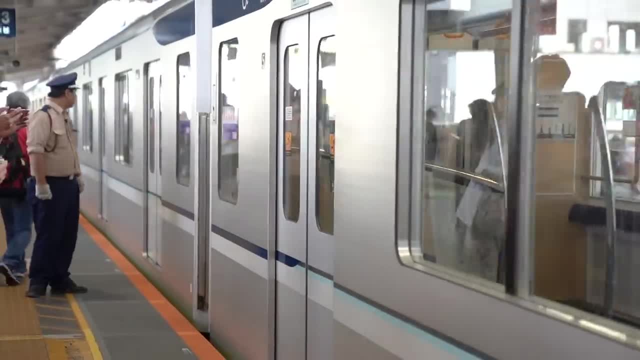 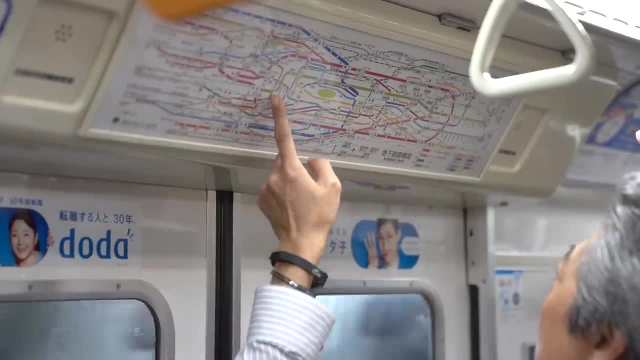 looking at this really complicated map very much. Something to note here is that Tokyo is not a driving city. There's certainly a lot of cars on the road, but for the most part people get around on the really smart public transportation system. This public transportation system. 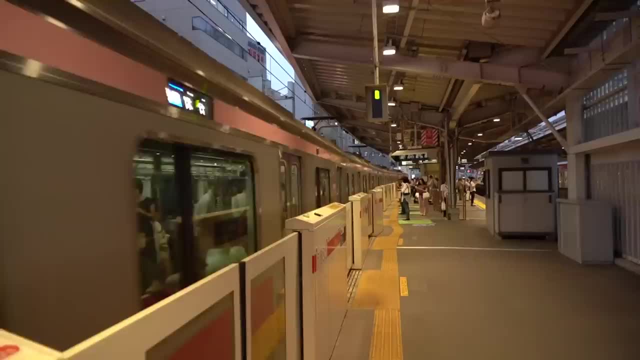 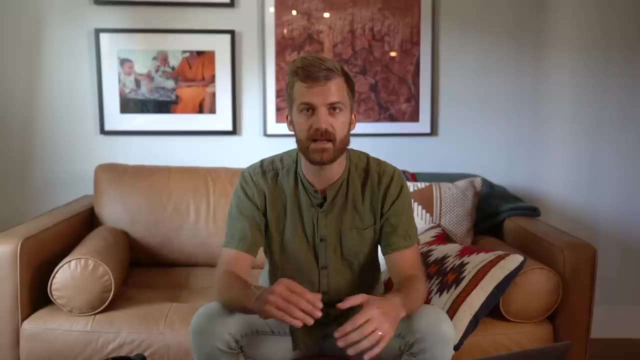 runs on mainly trains, which are some of the most efficient and on-time trains in the world. You will rarely wait a couple of minutes for a train, wherever you're going, at any time of the day, which makes transiting through Tokyo a very pleasant experience, if you know how to do it. 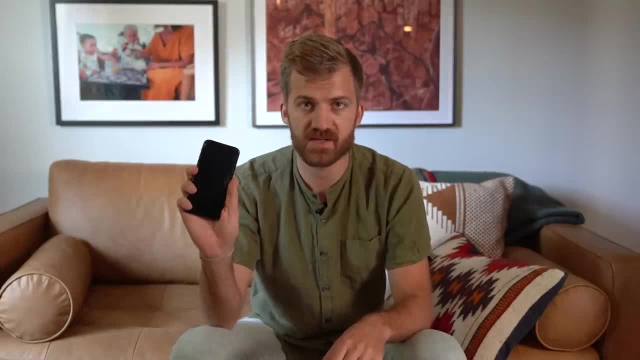 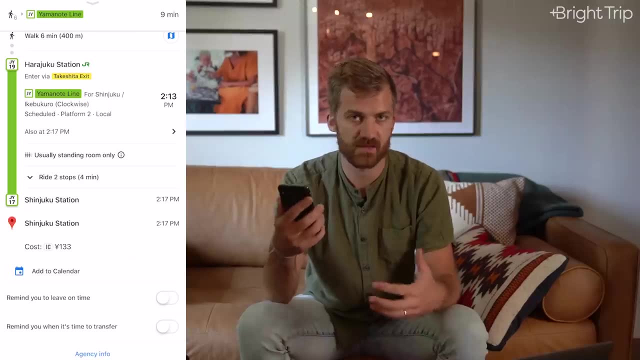 So, like I said, smartphone's going to be your best friend when using transportation in Tokyo. You can use Google Maps, which is what we prefer. It has real-time updates on when trains are coming and it's just a very easy interface. Another app that's really useful is called Tokyo Subway. 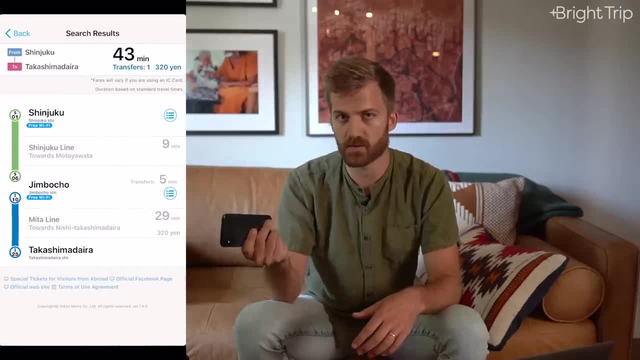 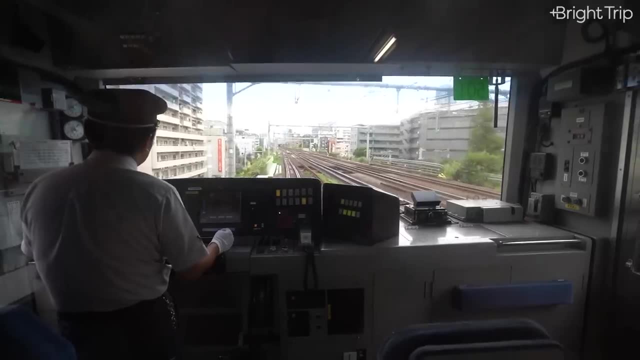 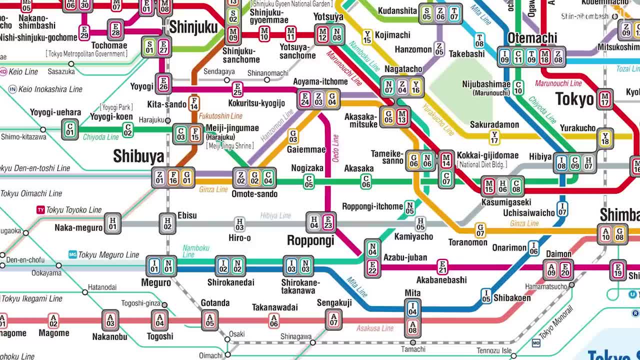 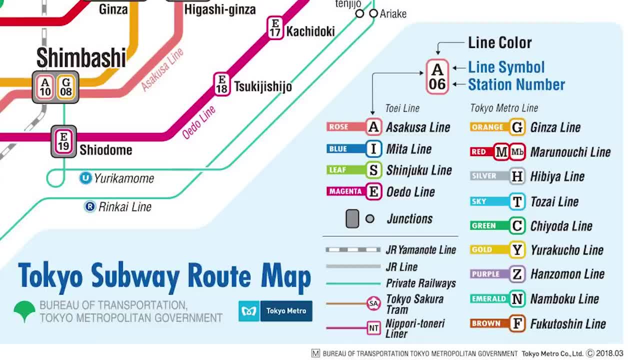 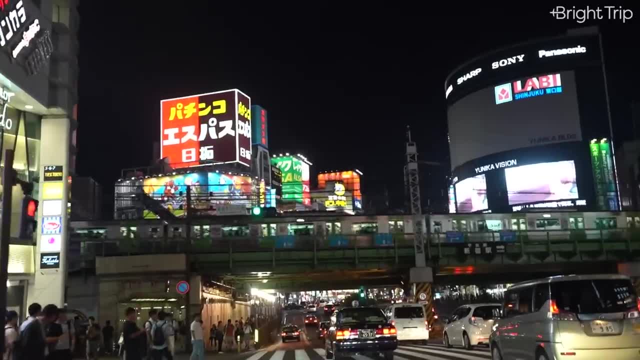 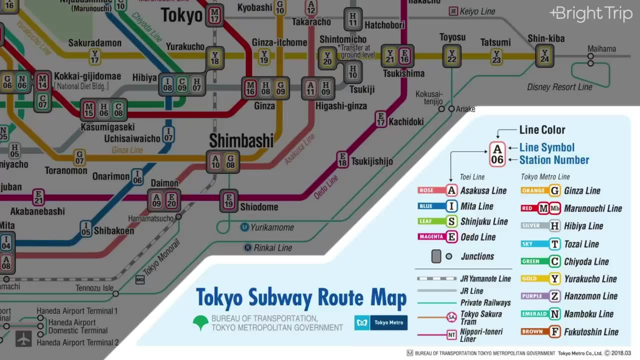 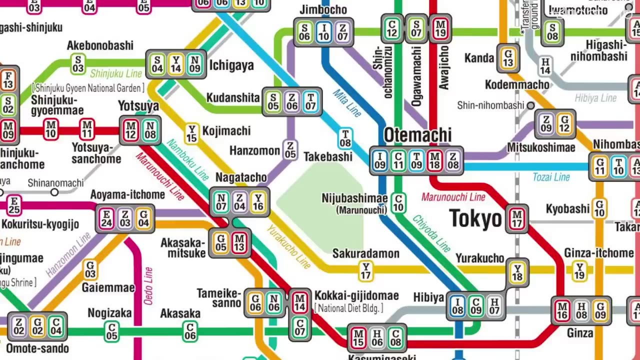 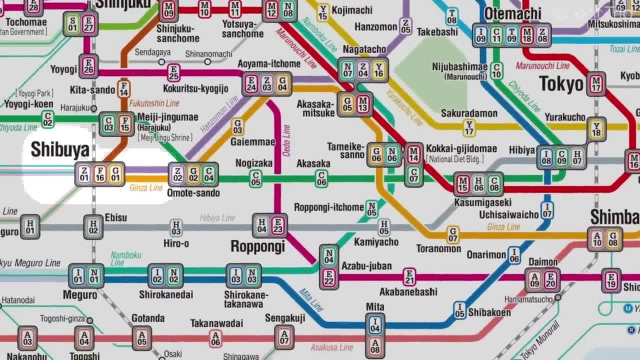 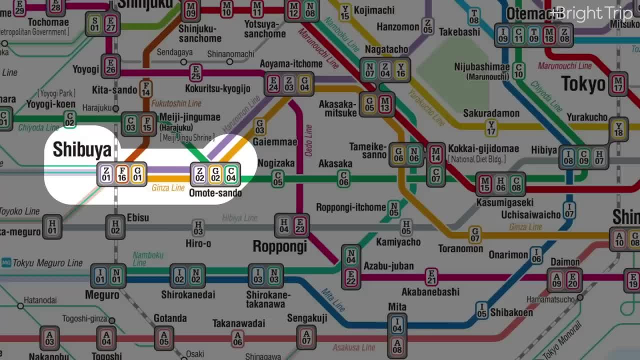 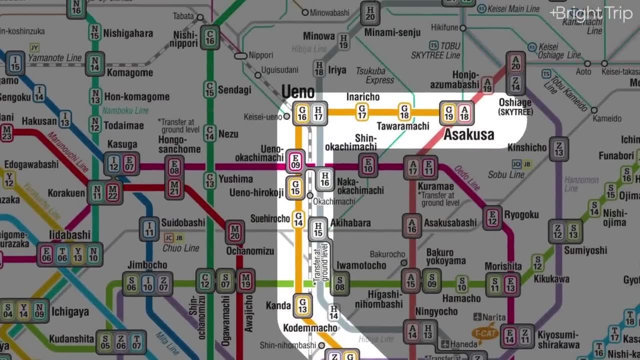 or down, depending on which direction you're going. So the Ginza line starts over here in Shibuya. You can see that this is number one. The next station is number two, and then number three and number four. This goes all the way until the very end of the Ginza line, which is number 19 out here. 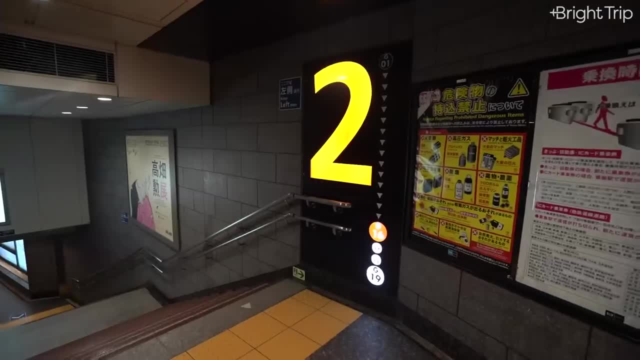 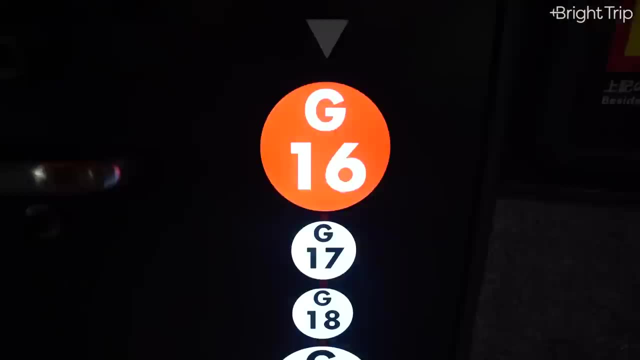 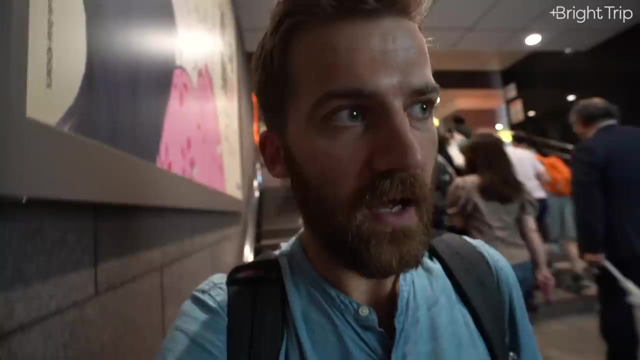 in Asakusa, Some stations will have these really useful little signs as you go down the stairs to the platform that tell you what the station number is- in this case, 16,- and what direction this platform is going. In this case, the numbers are going up to 17,, 18, and 19.. 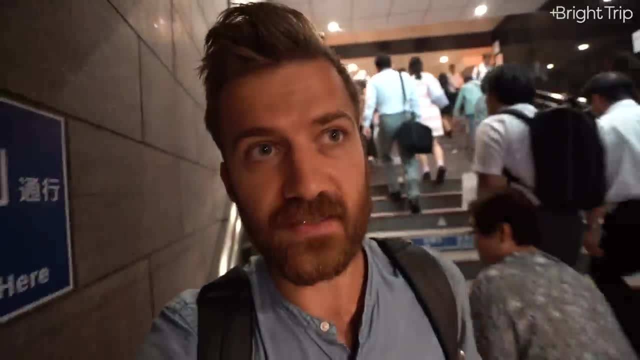 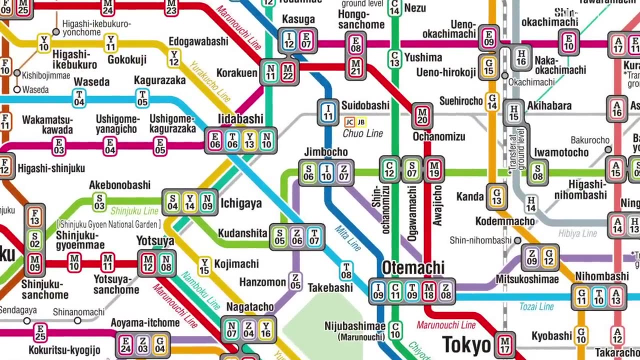 We're trying to get to 19 right now, So I know that this platform is going up. This is the right platform. Some stations have multiple lines that go through them, and so you'll see multiple numbers to indicate where, along the line, that station lies. 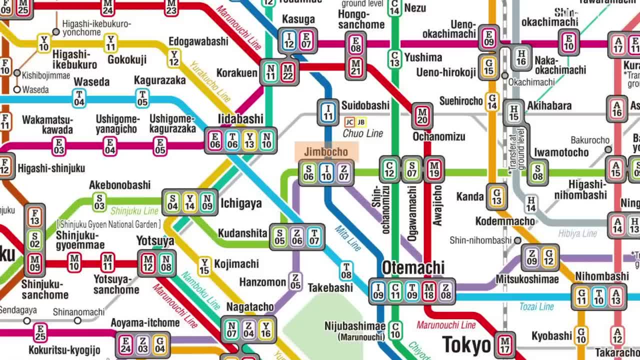 So, like this station called Jinbocho is the sixth stop on the green line and it's the tenth stop on the blue Mita line and it's the seventh stop on the purple Hanazonmo line. Okay, so don't get caught up on the fact that there are multiple numbers per station. 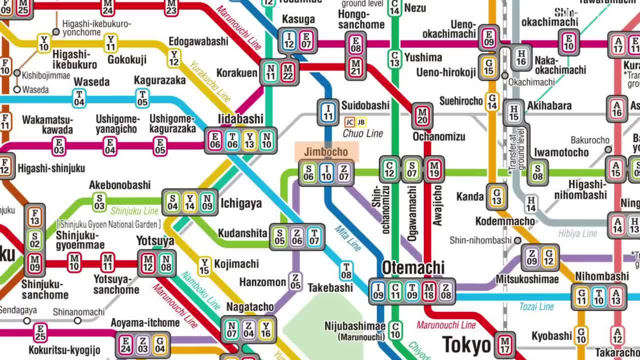 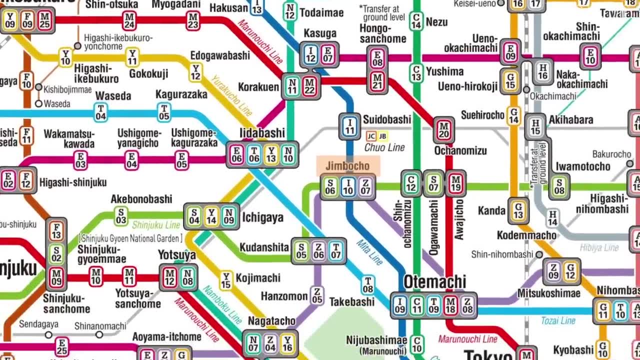 That's not important. What's really important Is to know that as you move along these lines, the numbers will either grow if you're going this direction, or shrink if you're going the other direction. The reason why this numbering thing is so important is because I don't know about you. 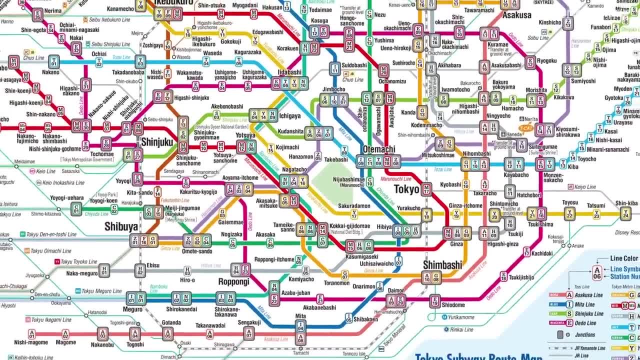 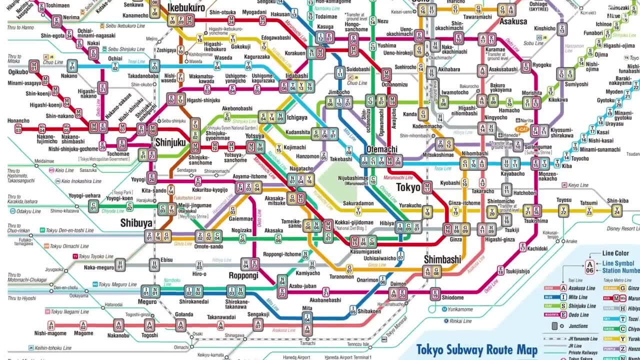 but for me it's really hard to memorize names in Japanese or any other language where the pronunciation is totally different than anything I'm used to. So, instead of remembering that you have to get off at the Shirokana Dai Takanawa station, 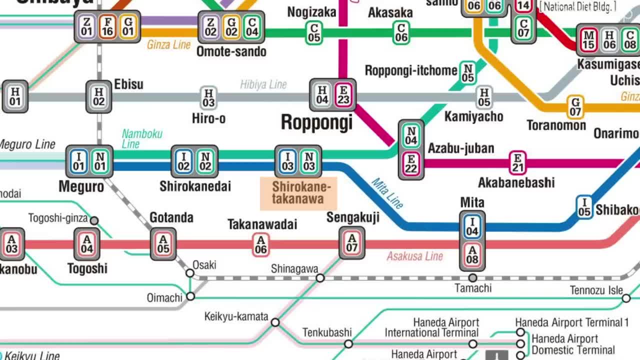 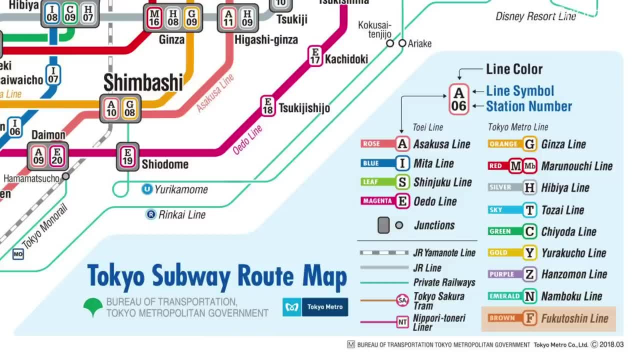 you can just remember that You have to get off at stop three when you're on the blue line. Same goes with the names of the lines themselves. Instead of trying to memorize the Fukutoshin line, just think of it as the brown line. 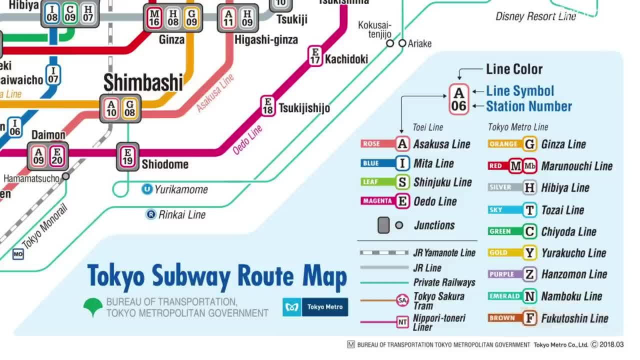 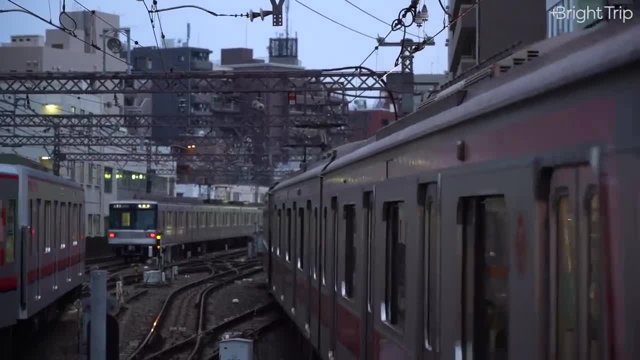 I'm sure the locals will laugh at you if you tell them you're thinking of it this way, but seriously, save the brain space for learning to say words in Japanese that actually help your experience, like arigatou, gozaimasu and konnichiwa. 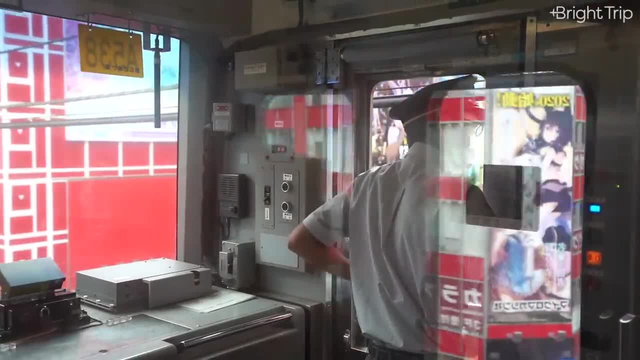 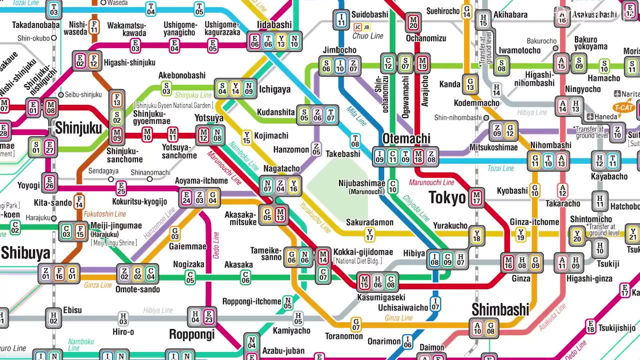 The names of the subways will only cause you stress if you're trying to memorize them. while you're on the train, You're zipping under the city and you're not sure where to get off. Okay, so we've come to the moment where we're done looking at this map. 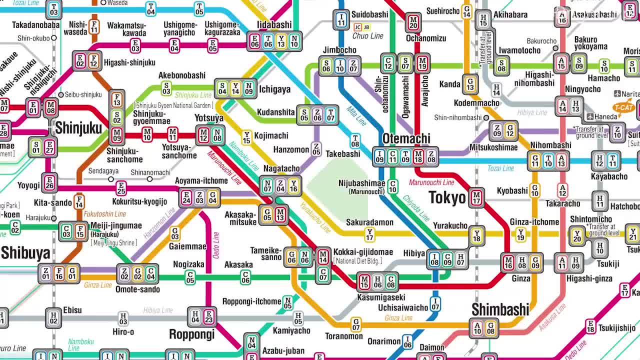 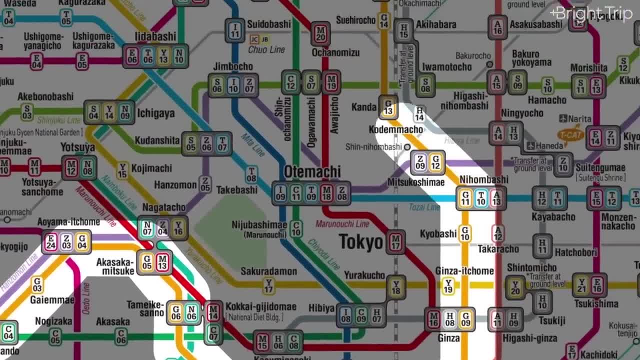 We only looked at it for one reason, and that's to know that each line has a color and each station along that line has a number that goes up and down depending on what direction you're going. This is the only information you really need to glean from this map. 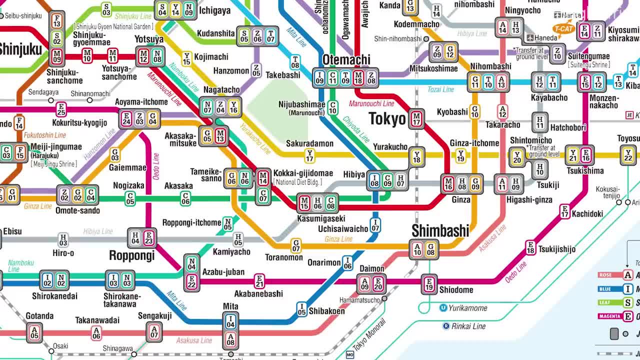 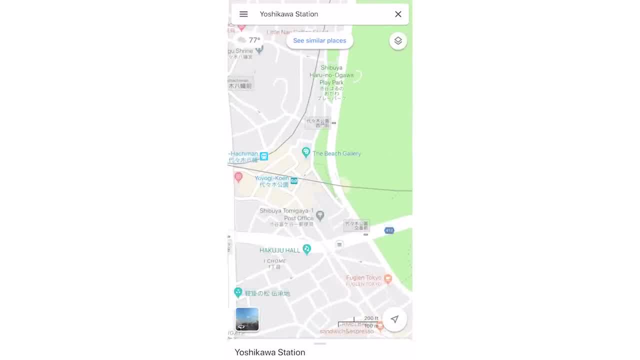 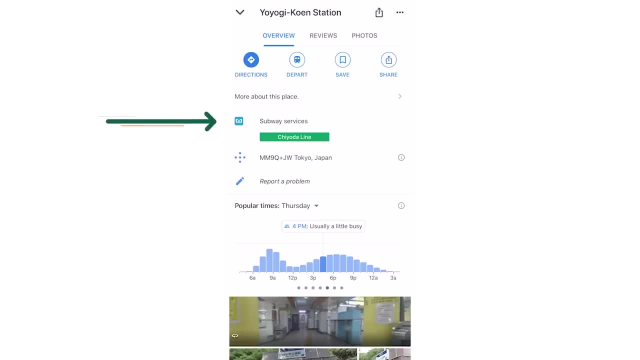 So let's talk about what it actually looks like to ride this train system. Often, Google will tell you how to get to the train station, where to walk, but you can always find them by looking at the symbols. M symbol represents the underground train, the metro, and this train symbol represents 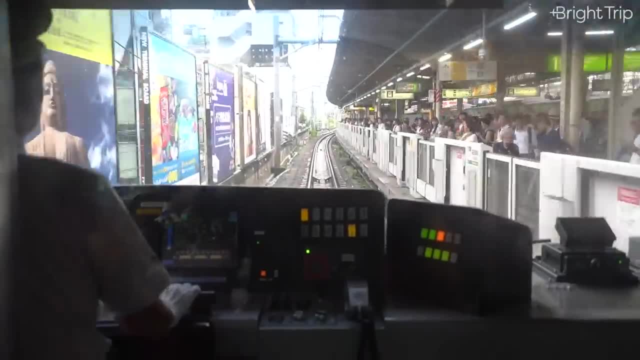 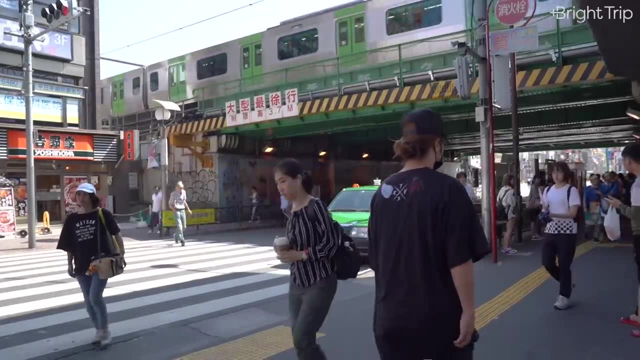 the above ground train. They function exactly the same and the card that you use is the same for both. You don't need to get too caught up in the above and below ground. They just have different symbols to indicate the different stations. Every once in a while you'll have to change trains by exiting the train station. 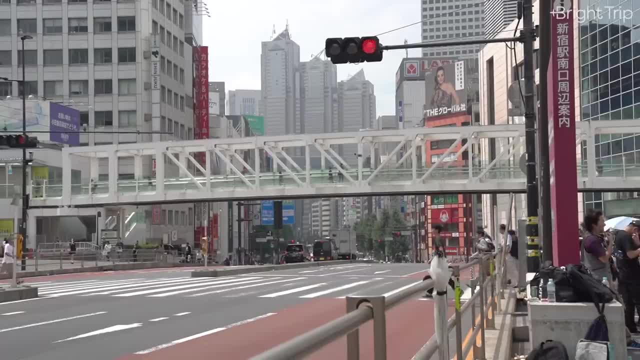 You'll have to change trains by exiting the train station. You don't need to get too caught up in the above and below ground. You'll have to change trains by exiting the train station. You'll have to change trains by exiting the train station. 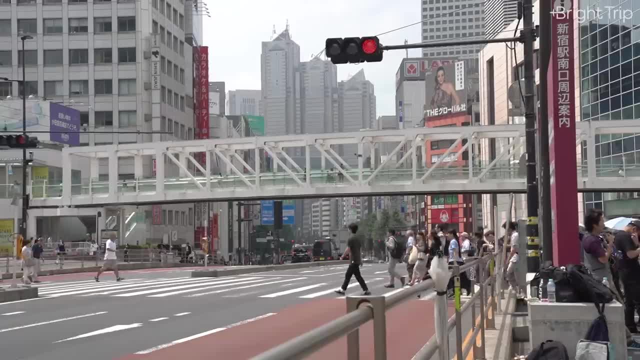 You don't need to get too caught up in the below ground station and going to an above ground station, But again, your app is going to tell you all of this, so you don't have to worry too much. Once you walk into a train station, you're going to see these. 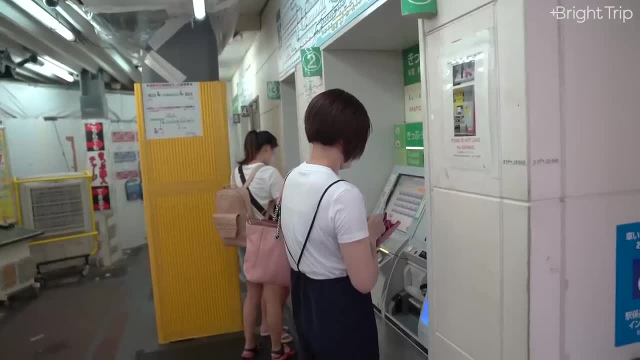 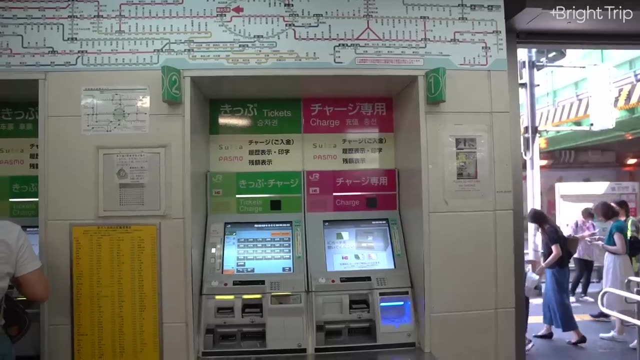 These kiosks are really helpful. It's where you get this one card that will make your life in Tokyo much easier. It's the card that we use for all types of transit in the city. There are two types of kiosks. 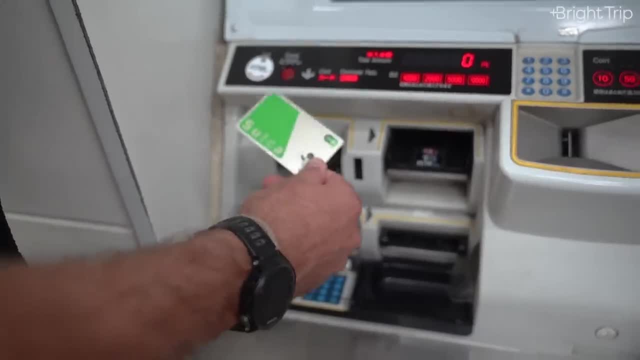 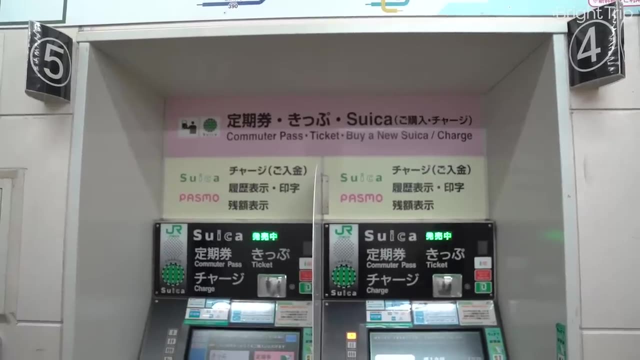 There are the kiosks where you can buy the card, and there are the kiosks where you can charge the card up with more money once the balance runs out, If you didn't already buy one of these cards in the airport. the thing you're looking for. 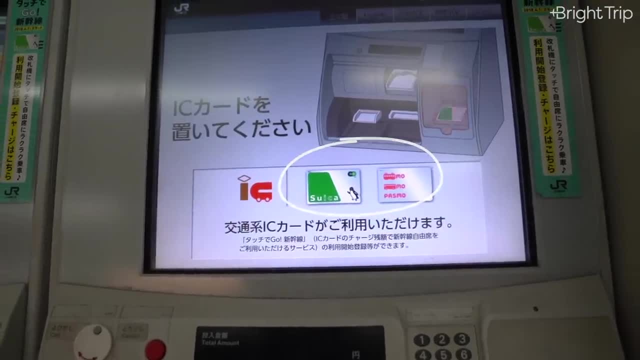 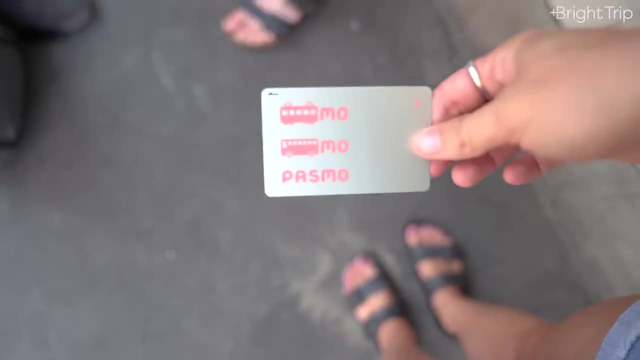 is this. There are two cards that do the exact same thing. They just happen to be from two different companies, So there's no difference. You can either get a Suica with this cute little penguin or you can get a PASMO with this. 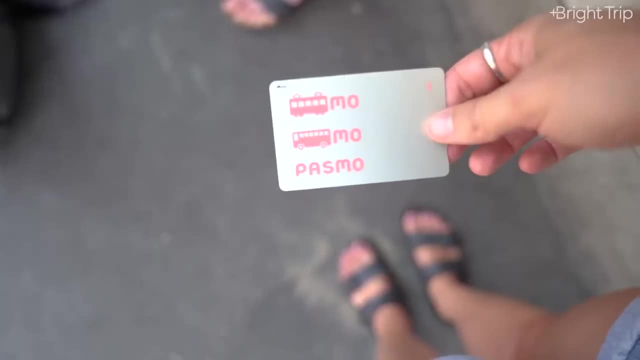 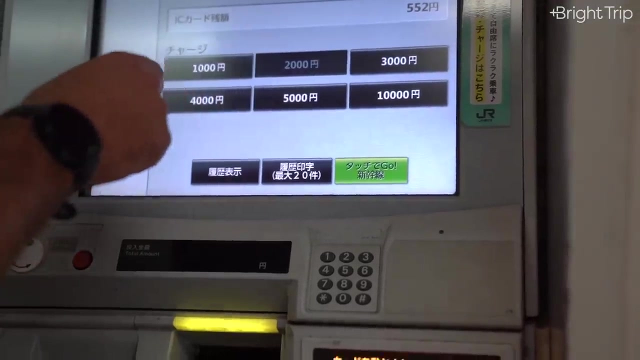 cool pink and gray color scheme. Totally up to you. So I follow the instructions to buy the card and it will ask me how much money I want to put on the card. Now. this will be a balance that I can use to ride the train. 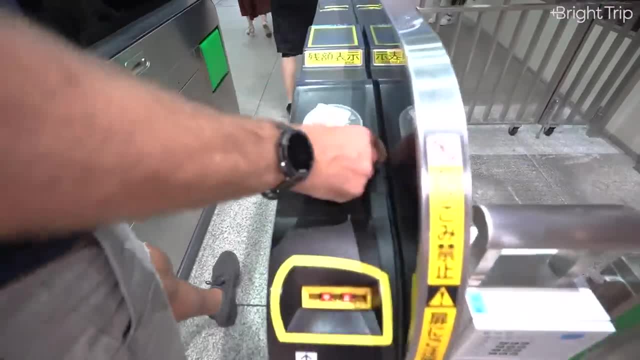 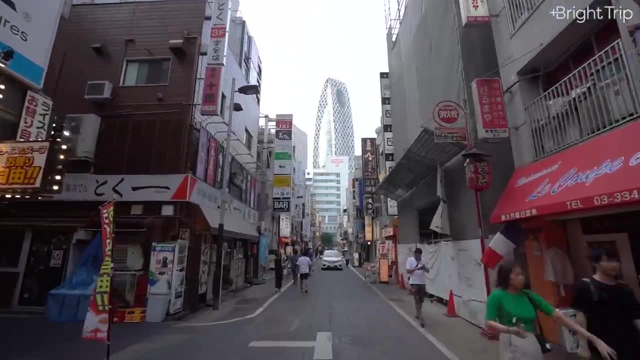 Every time I ride the train, I will tap in, I will tap out and it will take away a certain amount of money depending on how far I went. If you're going to be in Tokyo for a few days, I recommend putting at least 2,000 yen, which. 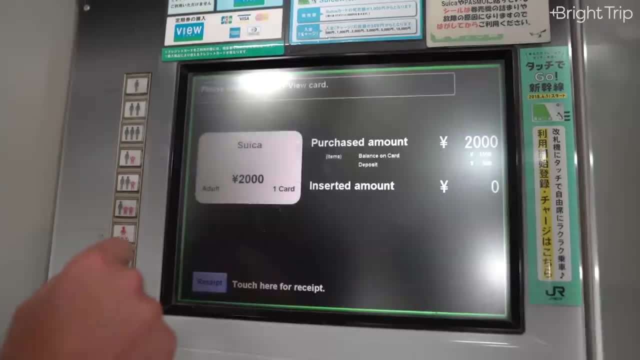 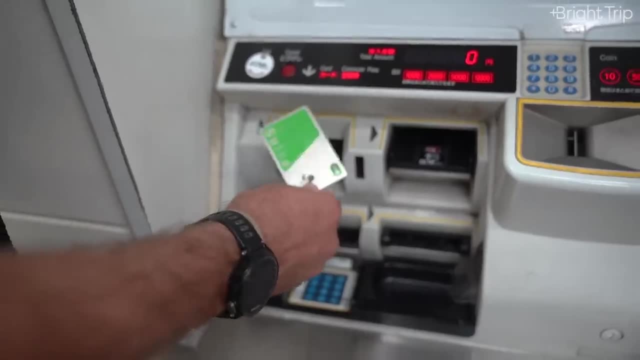 is approximately 20 US dollars to get you started, But if you're going to be there for four or five days or more, you might consider putting 5,000 yen on, which is around 50 US dollars, so that you don't have to go back and constantly. 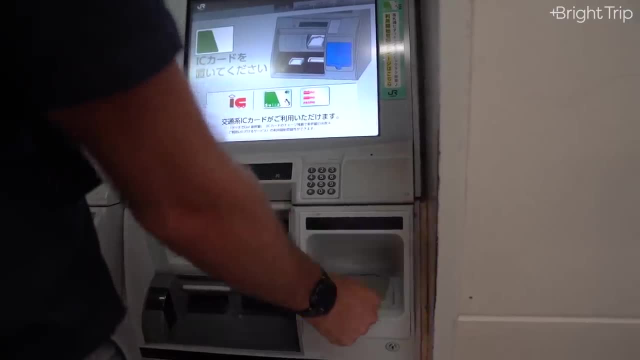 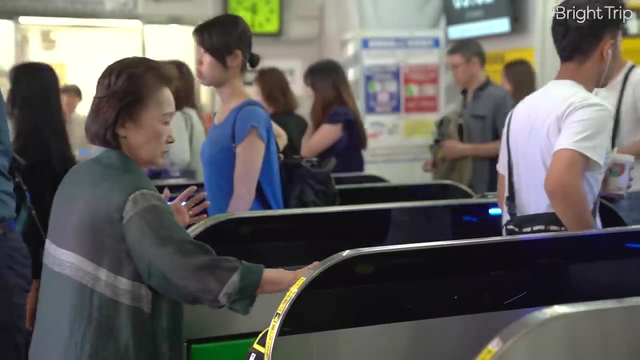 recharge. Speaking of recharging, there are kiosks everywhere to charge your card once it gets down to a zero balance, But you can check every time you go in and out of these gates. It'll tell you how much is left on your card. 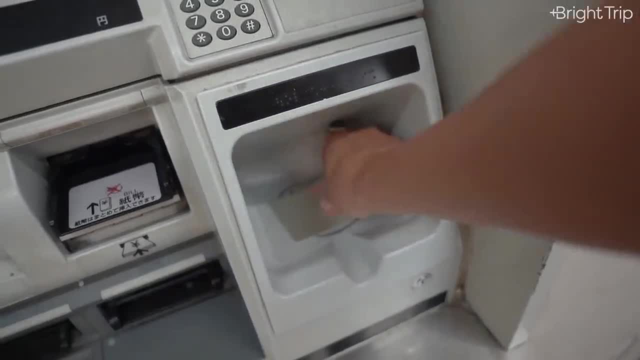 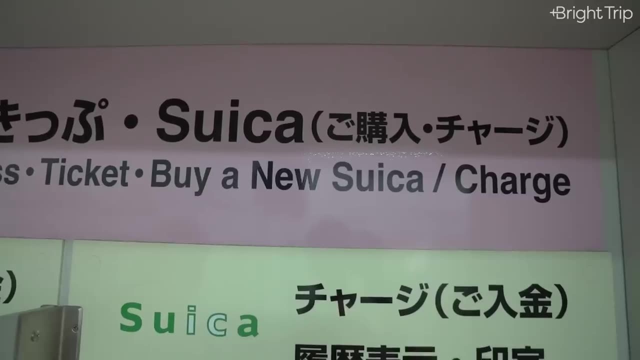 To recharge, you simply put your card in. It asks you how much you want to put on and you put the cash in and you're good to go. These machines only take cash, so be prepared for that. Just to buy the card, you actually put down a deposit of 500 yen or 5 US dollars. but 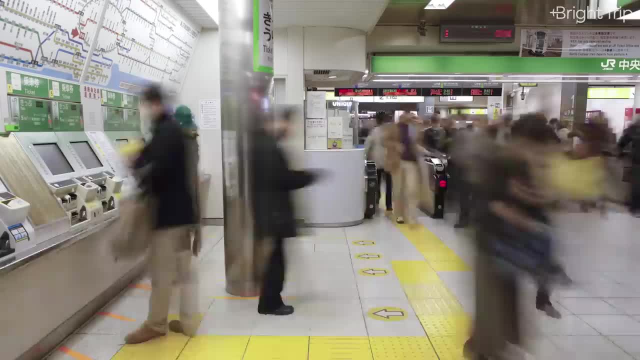 you can get that refunded when you go to an in-person ticket office on your way out of town and get that money back. So you've put your 1,000 or 2,000 or 3,000 yen in and you're ready to go. 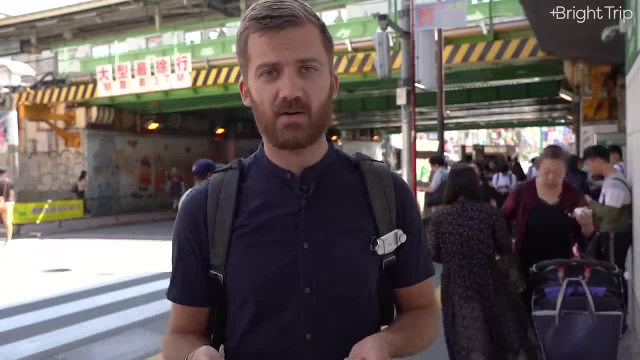 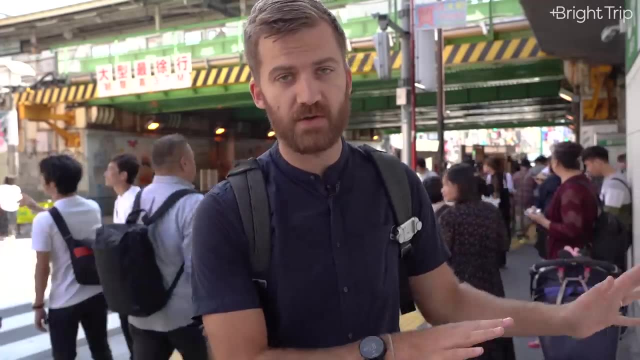 The card comes out and now you've got a PASMO card or a Suica card. These things are so useful, not just for riding the trains, which they're very useful for that, but for many other things too. Check this out. 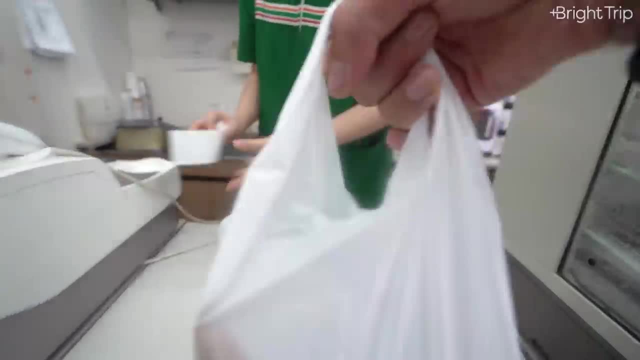 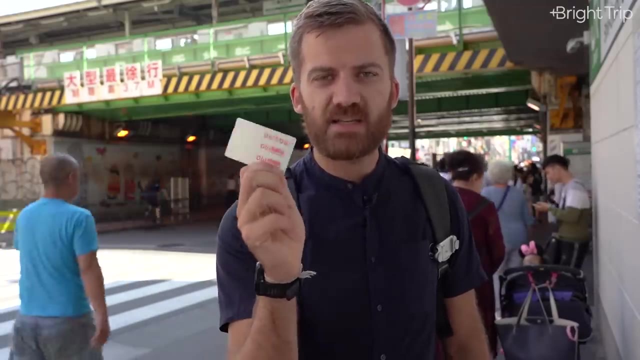 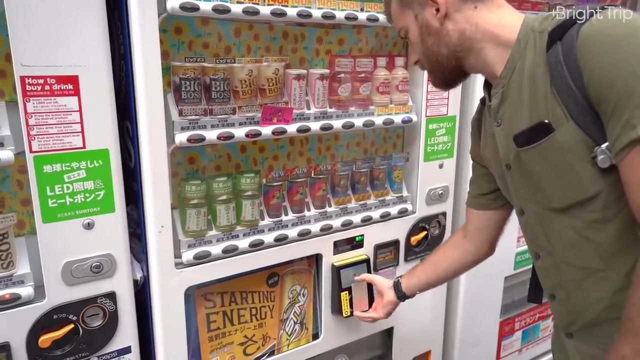 Yes, that's right. You can use this card and the balance you put on it at most convenience stores and even at some vending machines. It's amazing, It's like instant. You put it on to the little sensor and you've instantly checked out and you take your milk. 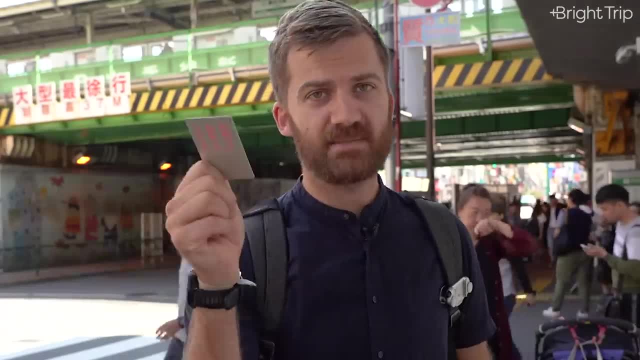 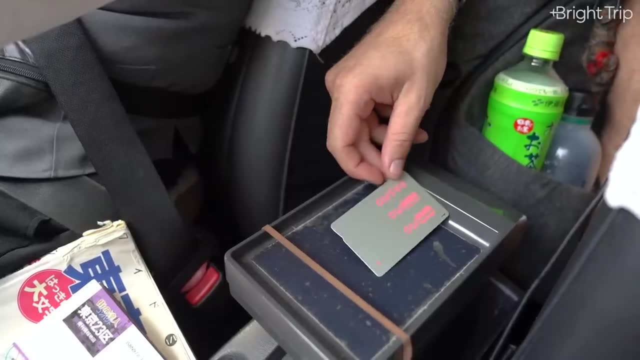 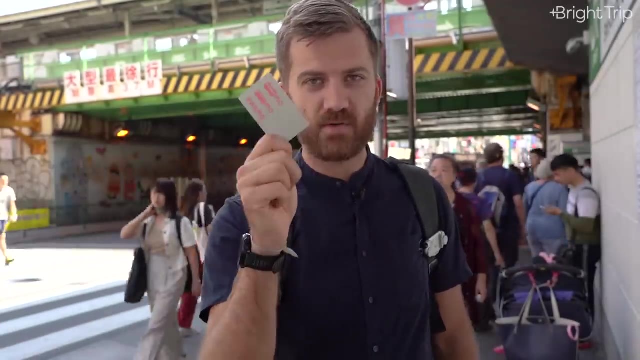 tea or sushi or whatever you bought, and you walk away. Oh and last bonus, the taxis in Tokyo now accept PASMO and Suica cards, so you can use this for taxis. This thing is seriously amazing, So make sure to pick up one of these, put enough money on it and use it wherever you. 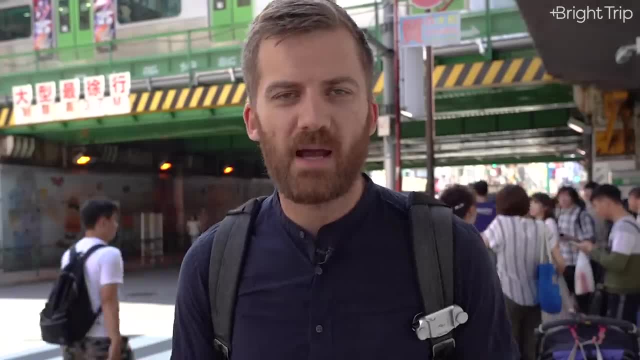 can, and you'll be amazed at how efficient it is. All right At this point. I'm sure it's still feeling overwhelming when you look at this. I'm sure it's still feeling overwhelming when you look at this, All right. 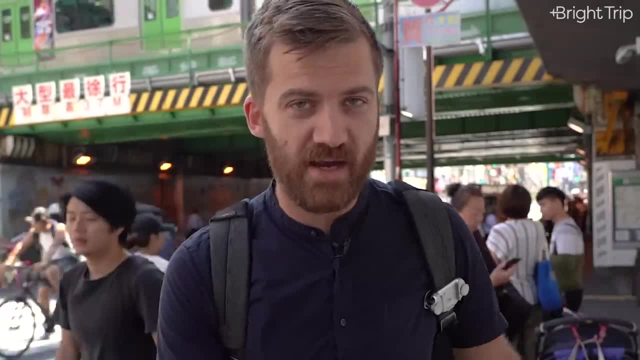 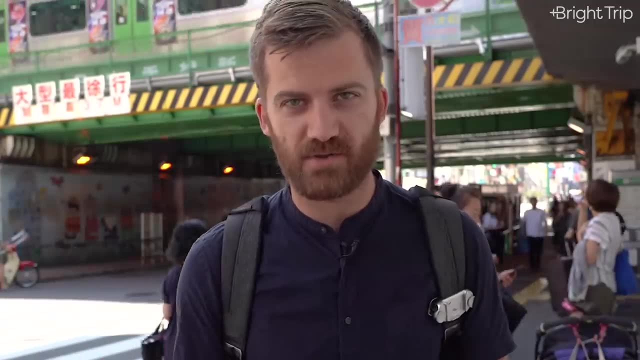 I'm sure it's still feeling overwhelming when you look at this map. Don't worry, We are actually going to go on and ride the train and show you each step of the way, so you know all of the concepts for riding from point A to point B on Tokyo's metro system. 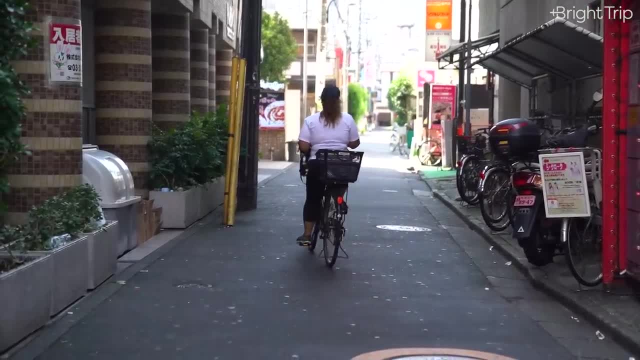 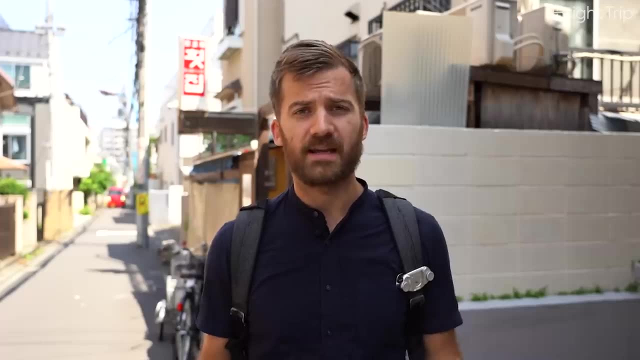 We've been spending the day here in Shinjuku walking around these quiet neighborhoods and we want to go into the center of Tokyo, to Tokyo Station, which is like the dead center of the entire city. We could take a taxi, but we shouldn't. 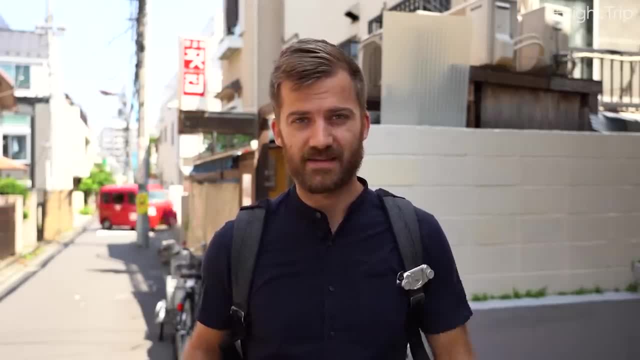 Don't take a taxi. This is not a driving city. This is a train city. This is one of the most efficient train systems on Earth, and you should really learn to take advantage of it so that you can get throughout the city in a seamless manner. 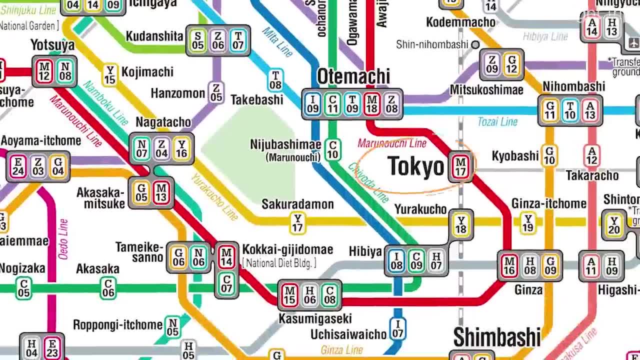 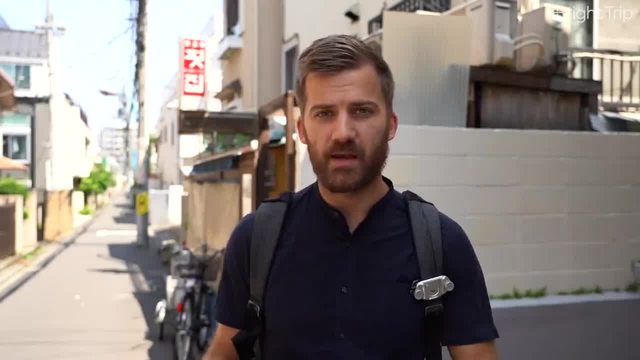 So we're going to show you how to do that- Get from Shinjuku to Tokyo Station using the wonderful train system. Before we jump on the train, let me talk about a few ground rules that you should keep in mind when getting around Tokyo. 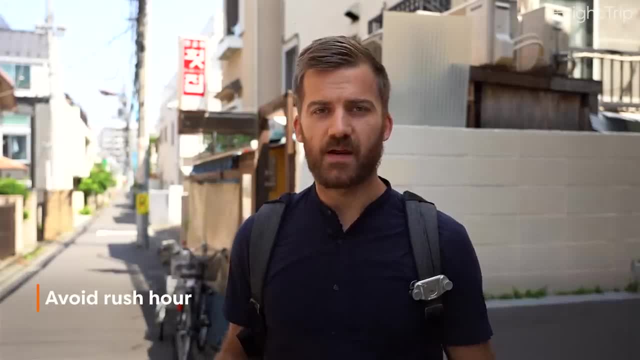 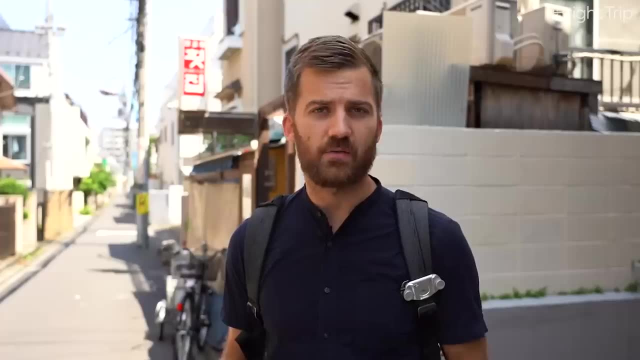 Number one: avoid the train during rush hour. Tokyo is a very, very big city. It's the most populous city on Earth and there are a lot of people who commute in and out of central Tokyo. Because of that, during rush hour, during peak times, like 10 am or 5 pm, kind of, 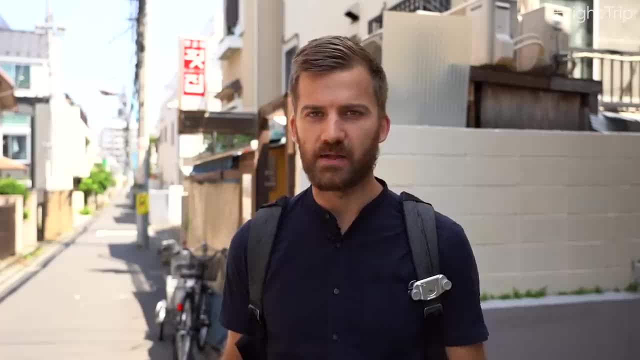 at the beginning and the end of the workday you are going to have really, really, really busy crowds. So if you can avoid rush hour, do it. It's not the worst thing in the world, and if you have to ride during rush hour, that's. 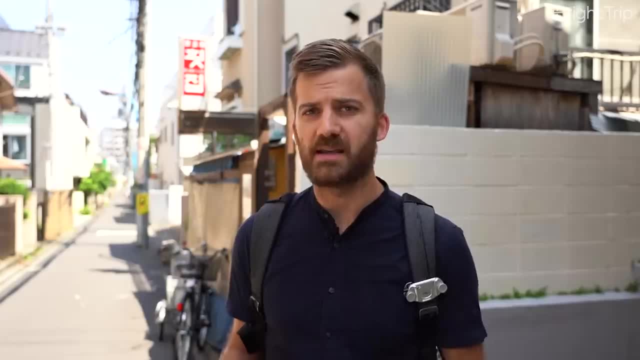 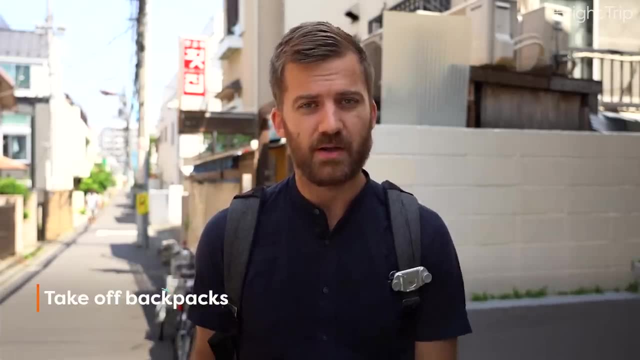 totally fine. But as a general rule of thumb, you probably want to avoid peak times if you don't want to be crammed with a bunch of other people. Next, it's kind of customary and good manners to take off your backpack and put it at your 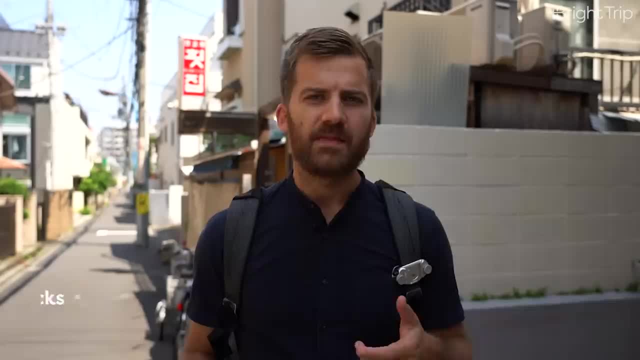 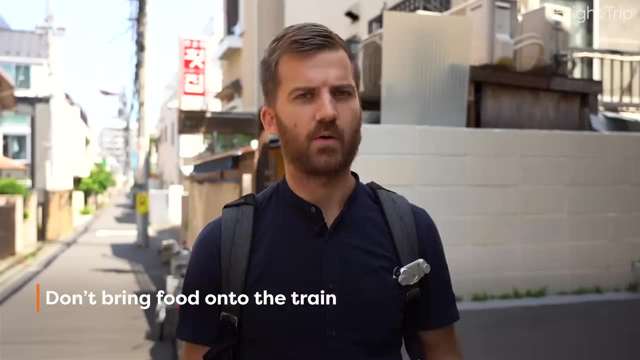 feet, so that you're not inadvertently crowding other people out when you're on them. The other rules are pretty ubiquitous among any mass transit system around the world, like don't bring food onto the train or if you see a disabled person or a pregnant woman. 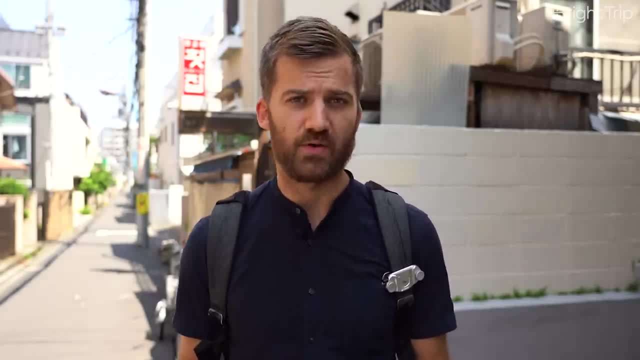 give up your seat, Things like that that are pretty intuitive, but definitely keep those in mind when you're riding the train here in Tokyo. Finally, we don't think that you have to memorize a ton of Japanese language terms to get around. 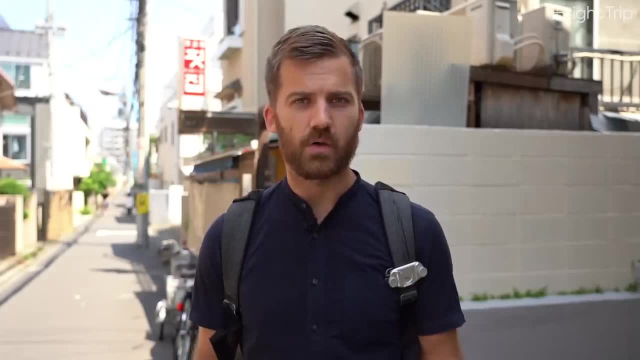 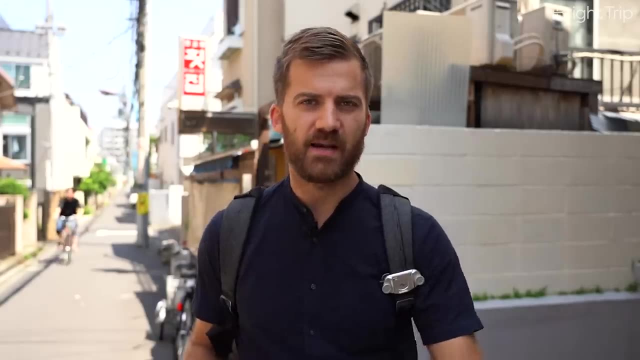 but there are a few that are just particularly useful, and one of those is the word sumimasen. Sumimasen means excuse me or sorry, or pardon me If you're on a busy train and trying to get to the door. if you just say a polite sumimasen. 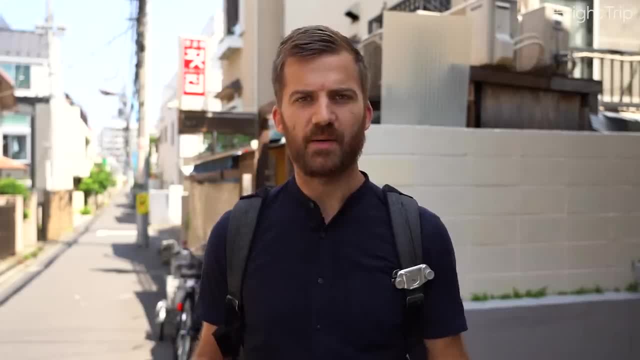 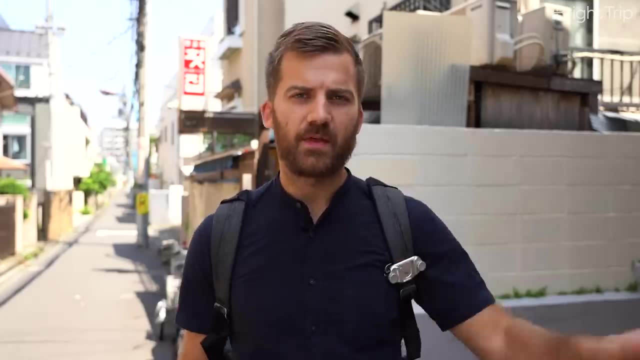 people will know that you're trying to get by and they'll move aside. So, sumimasen, it's an important one, It's one of a handful of phrases that we recommend you learn to kind of get around the city. So with those rules of thumb out of the way, let's actually start taking the train. 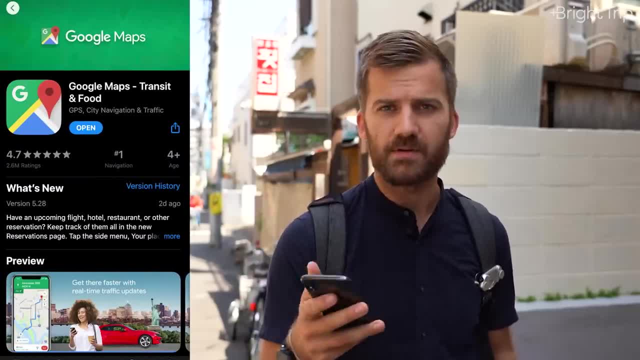 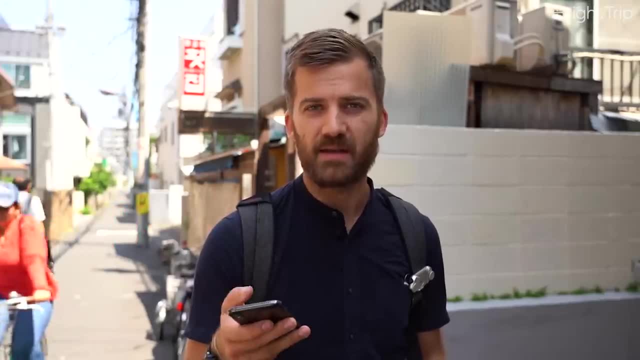 I'm going to pull up my phone. If you have internet, I suggest you use Google Maps. If you don't have internet, you can use the Tokyo subway app, which is available offline. Either way. what you're going to do is type in the destination that you want to take. 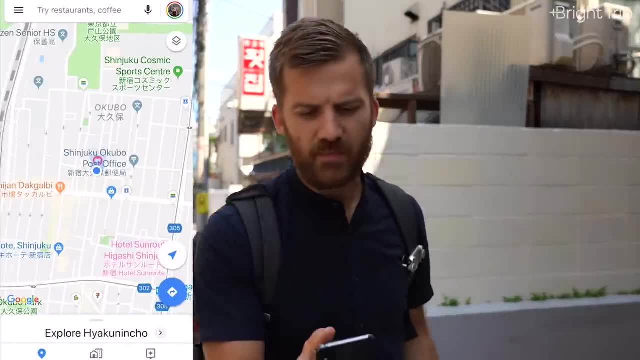 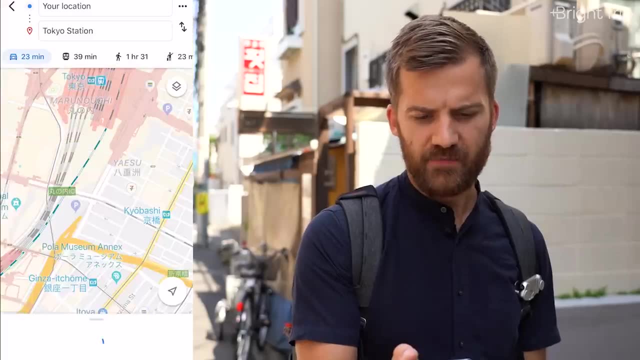 You want to get to. in our case, that's Tokyo Station. I'm going to open up Google Maps and I'm going to type in Tokyo Station, which is our destination, And then I'm going to hit directions. If it's on driving or walking, I'm going to make sure that this train icon is selected. 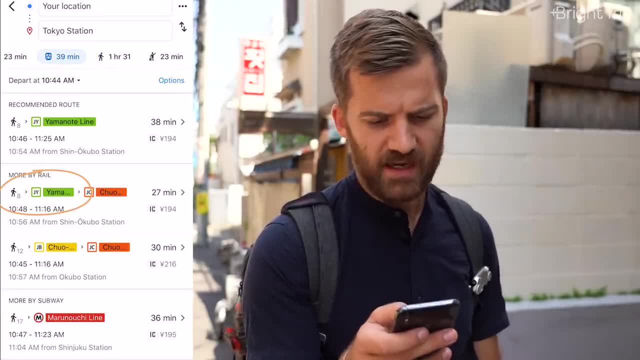 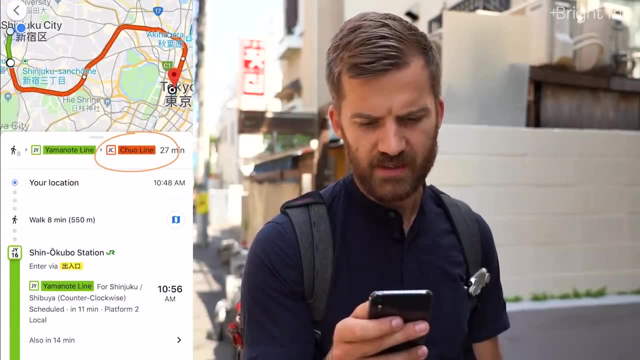 I'm seeing here that if I take the green line, which is J-Y, and then I transfer to the Chuo line, which is J-C, I can get to Tokyo Station in 27 minutes. I'll have to do one little transfer. 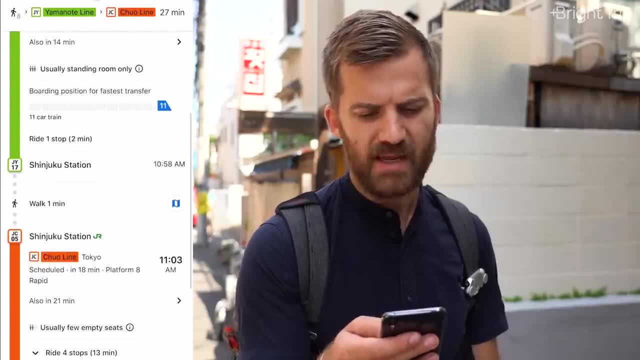 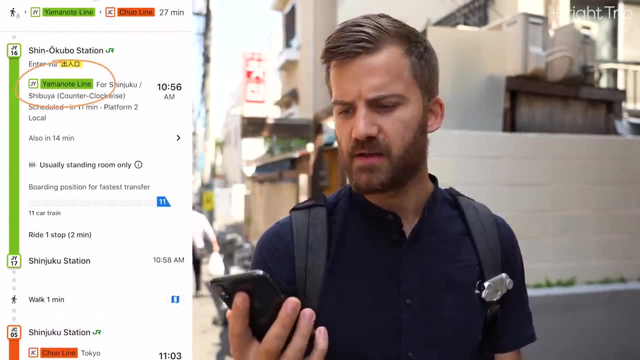 My whole itinerary is here laid out before me, and it tells me some pretty important information. The first really important piece of information that you have to look at when you're looking at your itinerary is the line that you're traveling. In this case, we're on this green line, which happens to be called the Yamanote line. 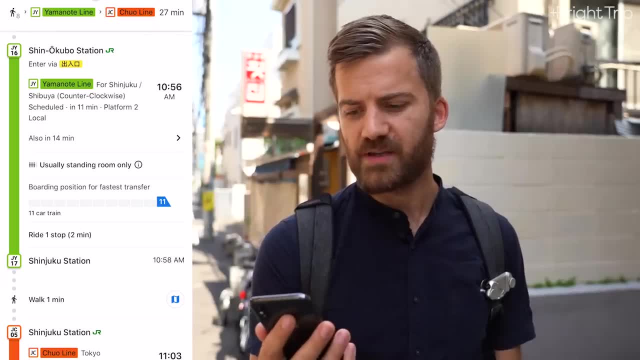 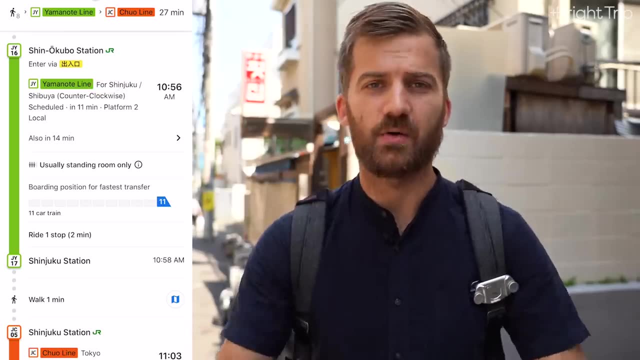 You don't have to know that, It's just the green line. The other really important information is the word for, For means which direction the train is going, meaning what destination it's going towards. So in this case, for Shinjuku. 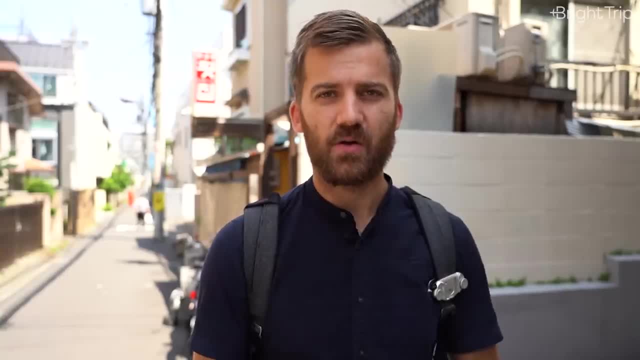 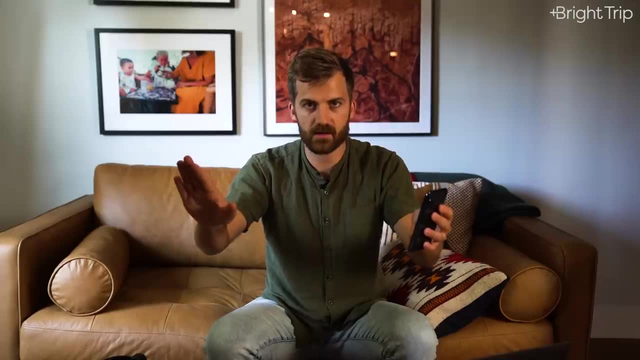 And Shinjuku For Shibuya Is the direction that it's going to be going and the signs at the station are going to reflect that. Whoa, whoa, whoa. Hold on a second Important caveat here, which is that sometimes in the app and even on the signage in the 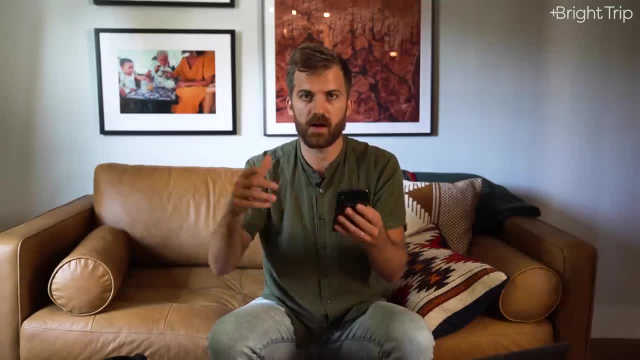 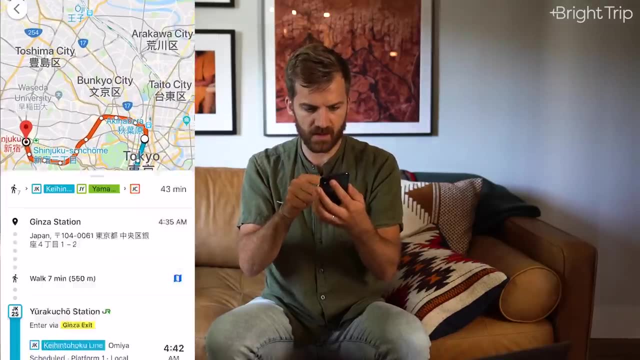 metro station- they're not going to use that word for- and then the final destination of the direction you're going. So I'm looking at this route right here. that tells me that I'm going on this blue line from station 25 to 27.. 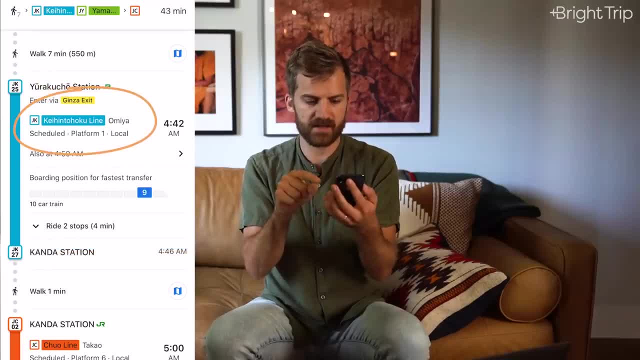 And I'm taking the blue line Towards Omiya. It's not saying for Omiya- which would be really nice if it did- It's just saying Omiya. This, even though it seems kind of hidden, is really important. 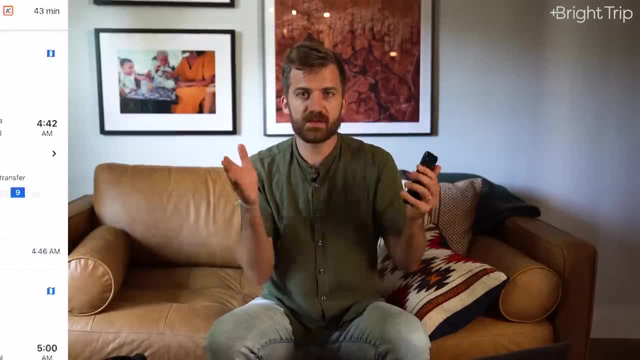 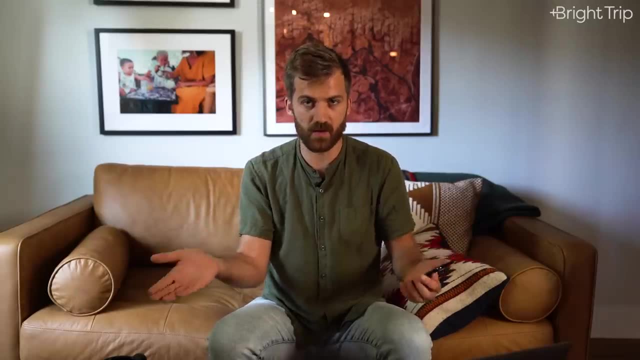 It's always to the right of the line that you're taking. This really matters because if you get on the right line but going in the wrong direction, you're not going to end up where you want to be. So you need to look to the right of the line to see what direction the train is going. 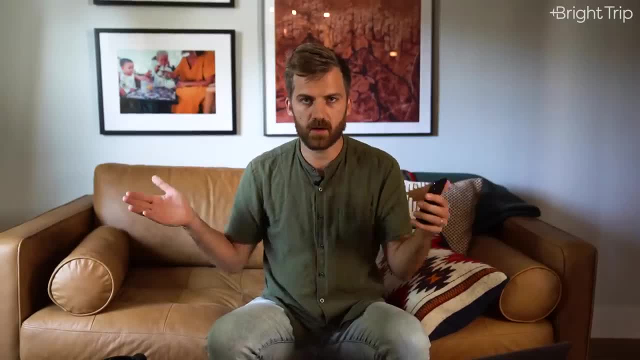 Sometimes it's followed by four. Oftentimes it's not All right Back to Tokyo, so we can see what this looks like. So when I get there, I can get to the green line and it can take me two different ways. 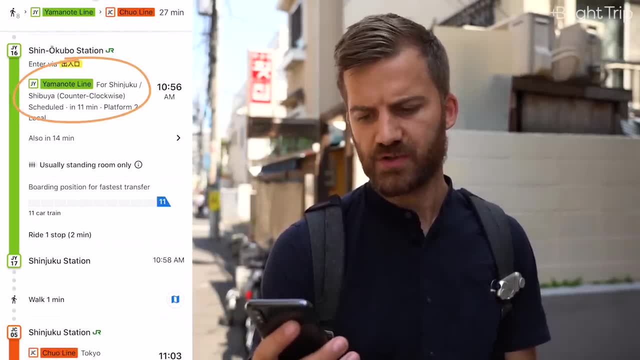 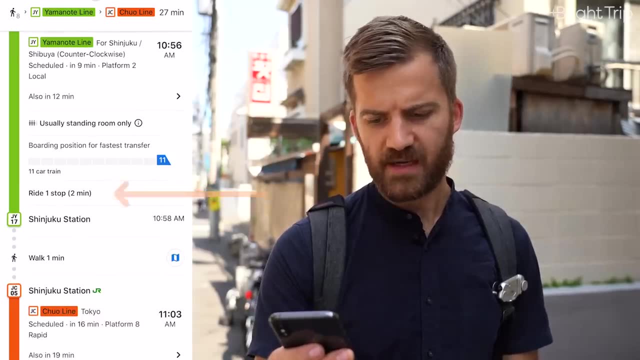 I want to get on the platform that says for Shinjuku and Shibuya. That's really important. If you get on the wrong platform, you'll go the wrong way. It's going to have me take it for just one stop. I'm going to get off at Shinjuku station. 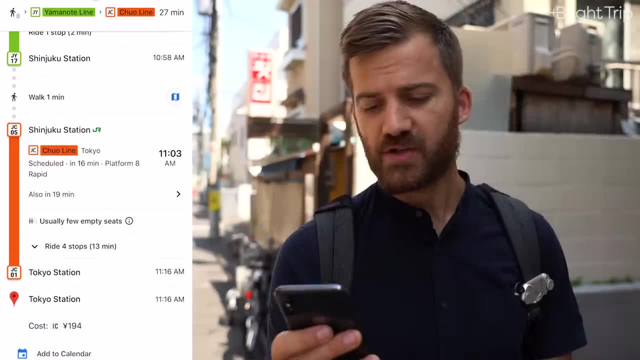 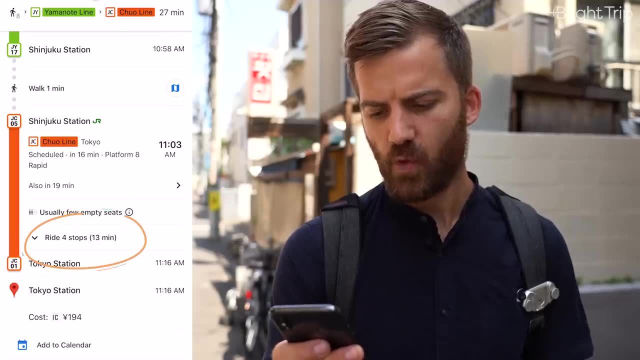 So from there I can see that I walk to the Chuo line. I want to make sure that I'm on the platform that's going towards Tokyo station- In this case it just says Tokyo- And then I'm going to ride it for four stops, which is 13 minutes, and then I will have arrived. 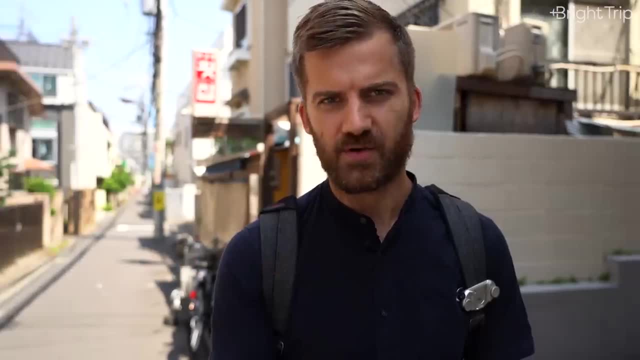 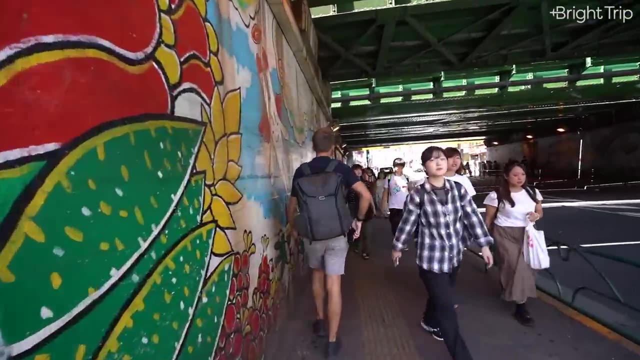 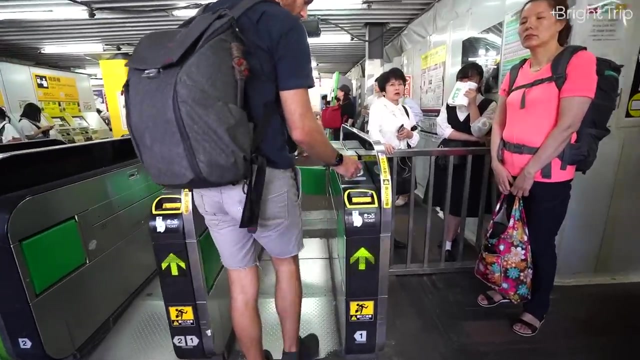 at Tokyo station. That whole journey will take me 27 minutes- One simple transfer. Let's go see what this looks like in real life. All right, So we're at the metro. We get into the entrance, We use our PASMO or Suica card to tap in. 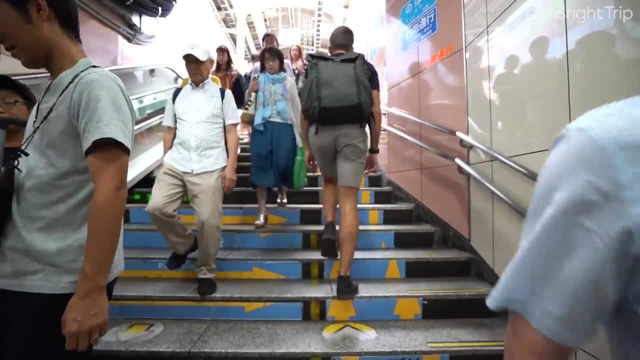 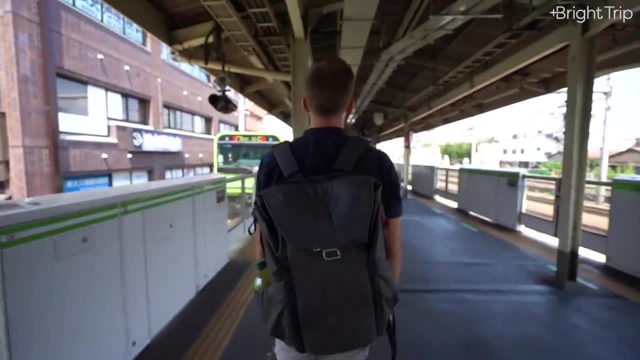 And now we're inside of the train station. So I'm looking for signs that say, just like my app told me, the green line for Shinjuku slash Suboya. Here it is, Following the signs and going to the platform that it indicates. 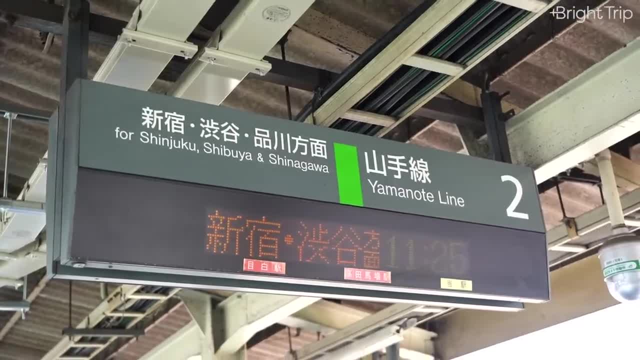 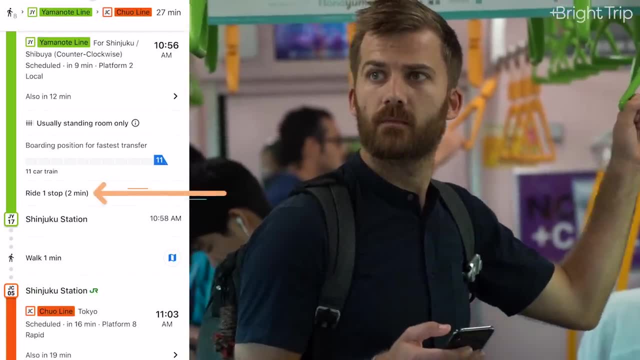 We're now on the platform and we wait. You can look up at these really nice signs that tell you when the next train is. The train comes. We get onto the train and we ride it, as my app tells me for one stop, to get off at Shinjuku. 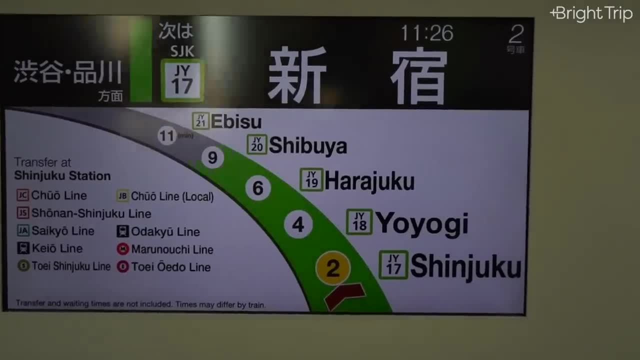 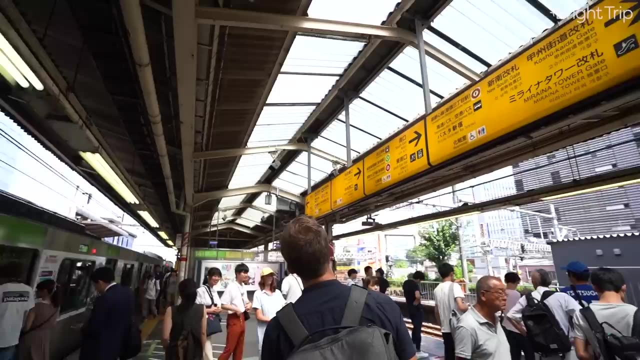 If you're into the numbers thing, like we explained earlier, I'm going from station 16 to station 17.. One stop: We're at Shinjuku. It's time to get off. We get off the train And now. 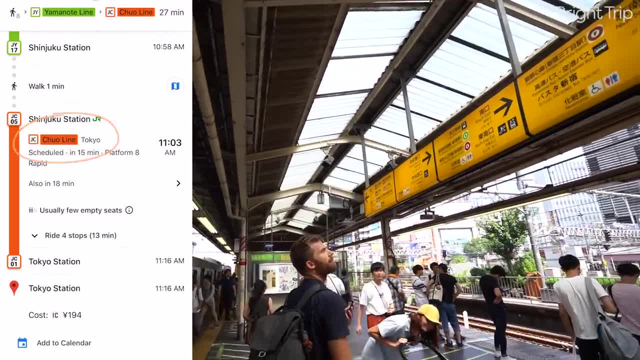 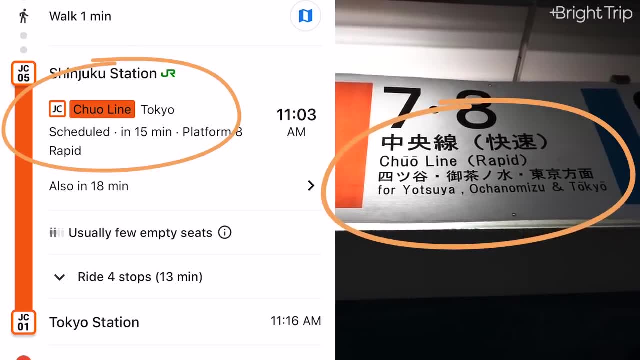 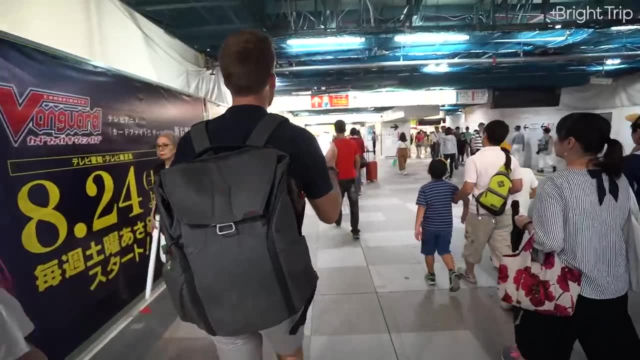 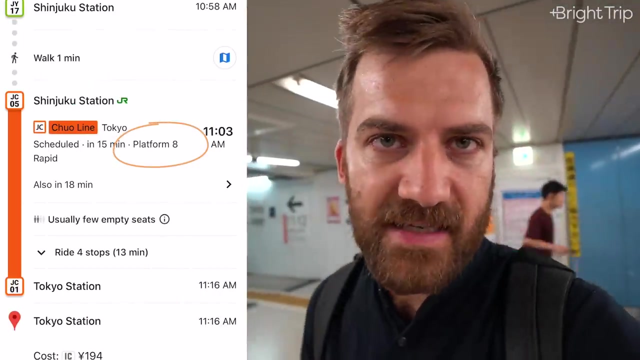 We're going to our app. We need to find this Chuo line. Luckily, the signs that point you where to go are everywhere, And there it is. We're going to the Chuo line for Tokyo Station. The other thing you can look out for on your app is the platform number, if that's easier.